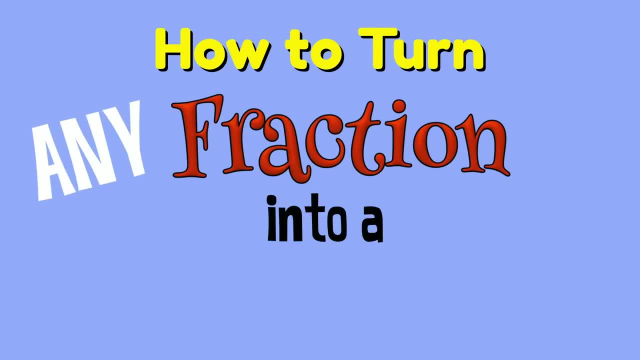 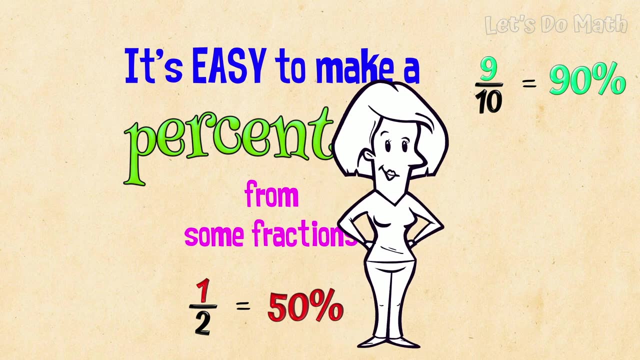 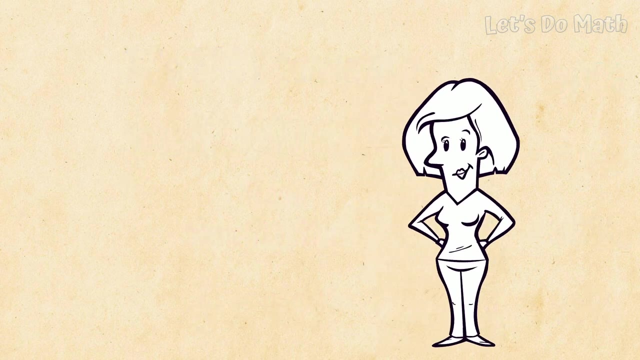 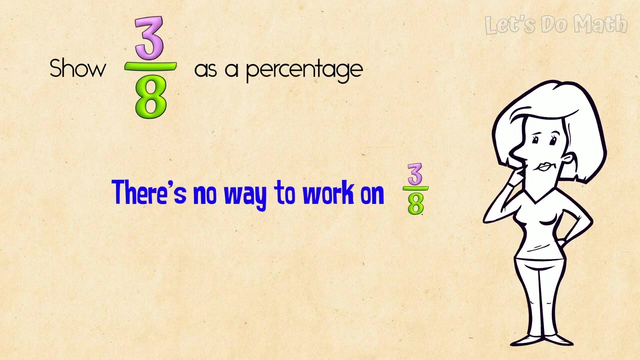 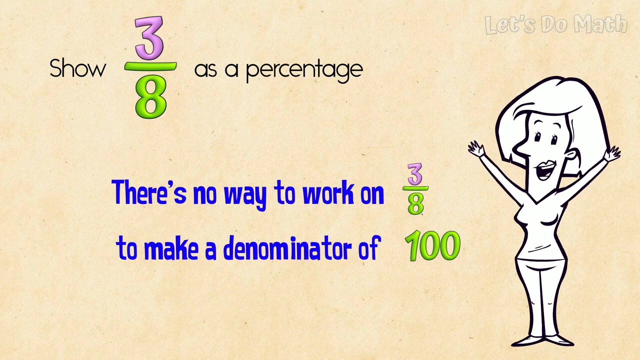 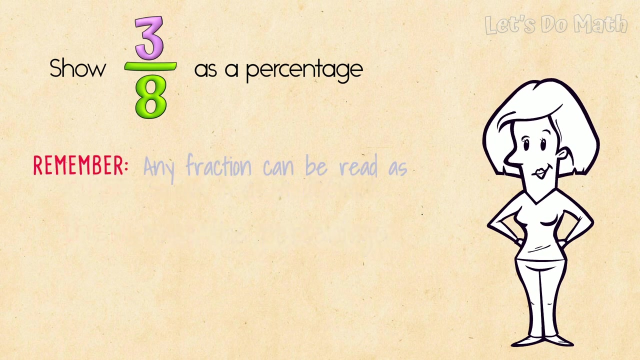 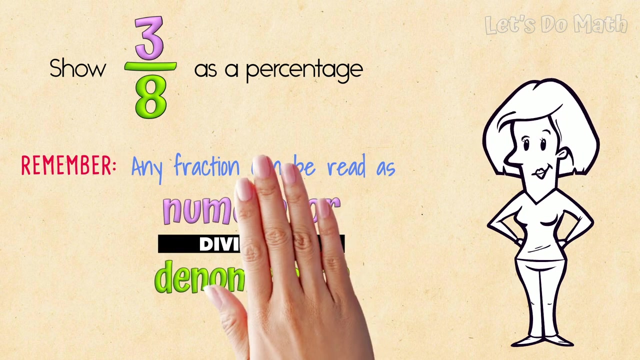 How to turn any fraction into a percentage. You can handle this one too. First we have to show it as a decimal, And from there we make the percentage. Remember, any fraction can be read as We want: 3 divided by 8.. 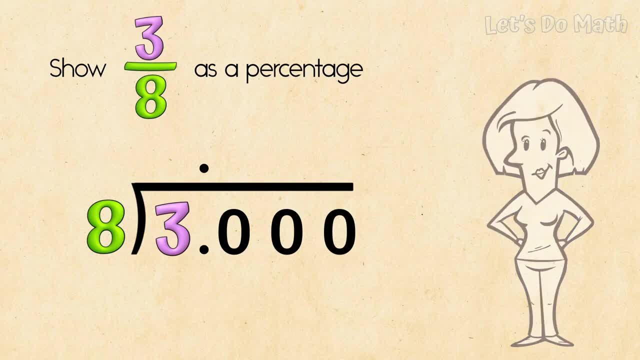 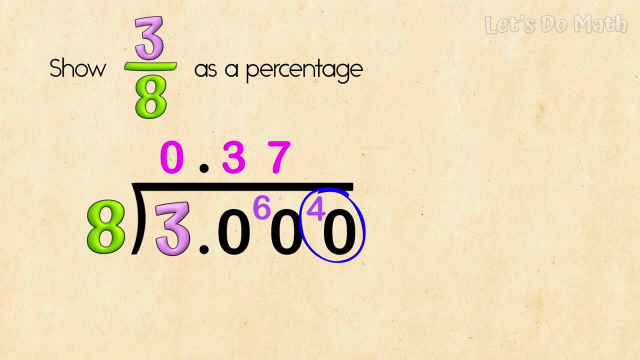 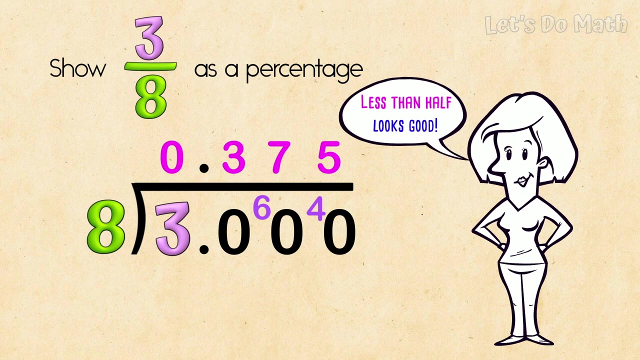 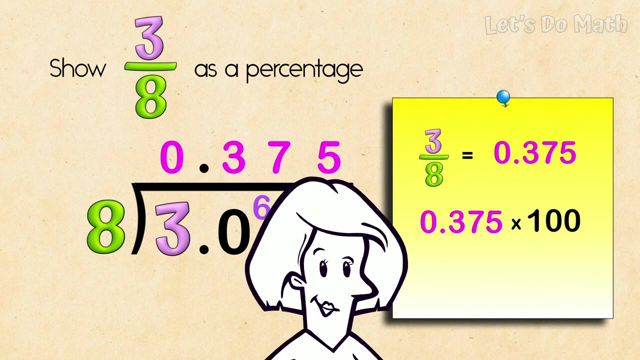 I'll need a decimal point and some zeros here And of course, if you're allowed, a calculator. that just makes things faster. So now we've got a decimal value. we make a percentage from that. We just multiply it by 100. 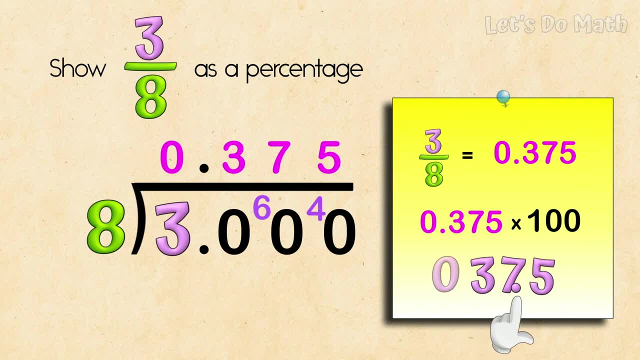 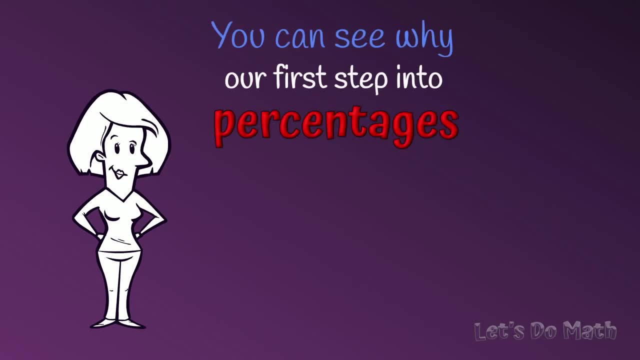 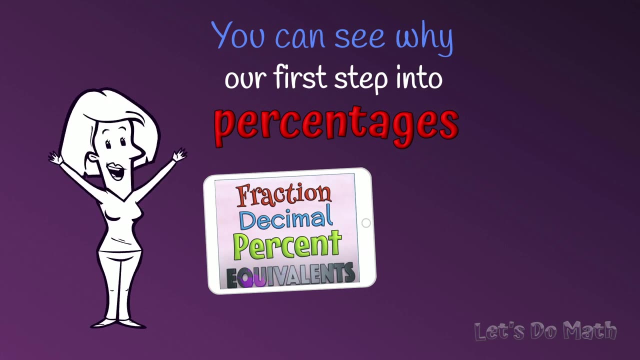 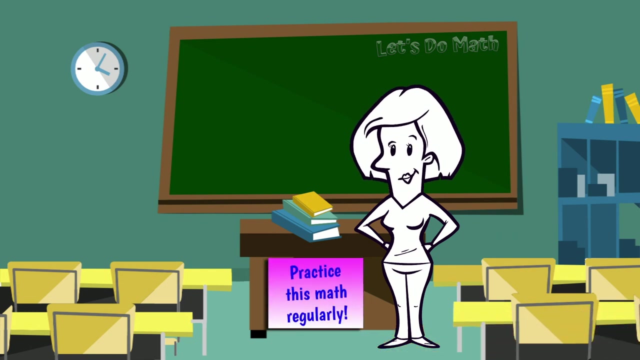 375 becomes 37.5%. You can see why our first step into percentages was all that practice turning a fraction into a decimal and a percent amount. This is a skill you really need in your math toolkit. If you're lucky, your teacher will get you practicing this regularly. 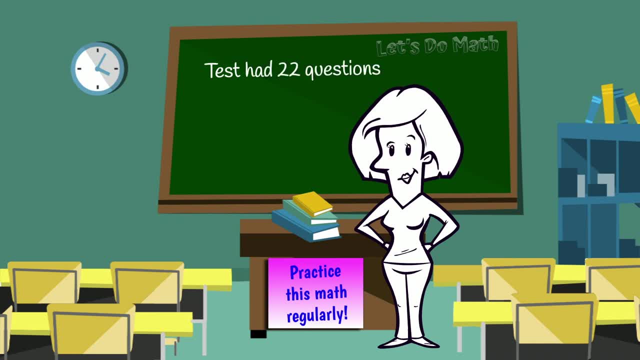 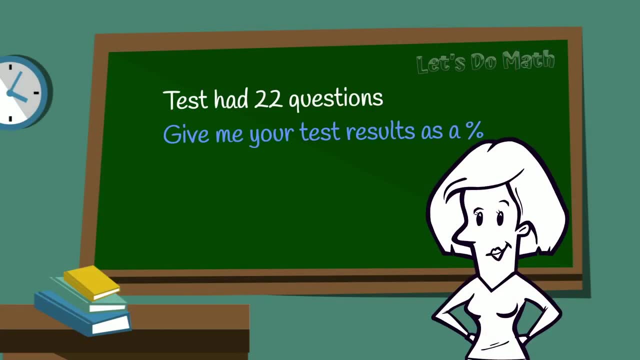 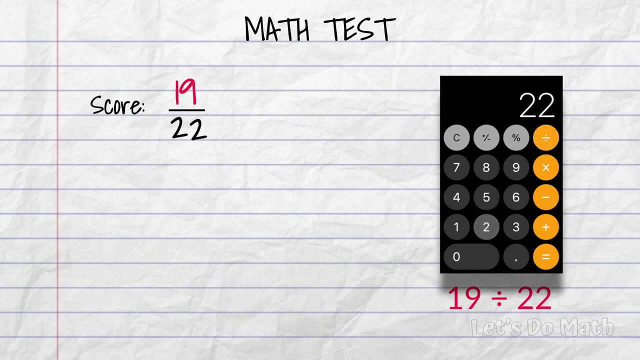 You could have a test with 22 questions And let's say you get 19 right. The teacher says: Give me your test results as a percentage. You pull out your calculator and confidently go: 19 divided by 22: 0.8636 recurring. 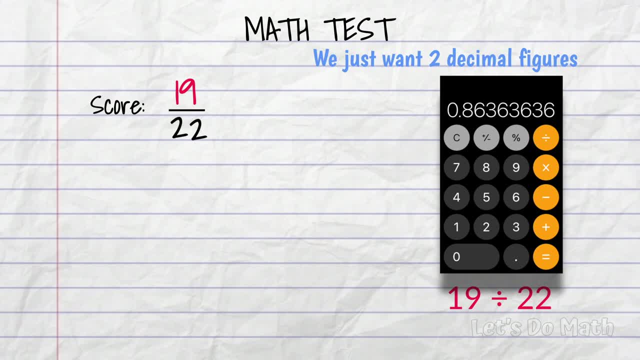 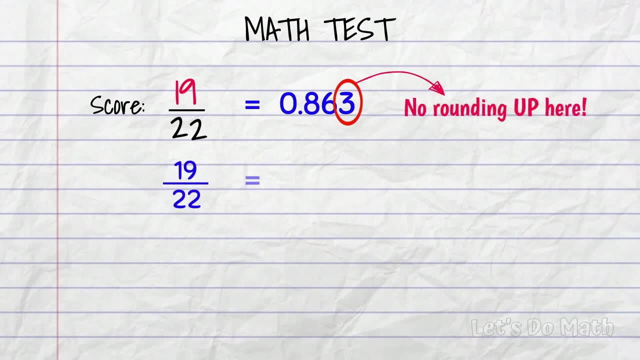 Well, we just want 2 decimal figures. The third figure tells us what to do. It's a 3, so no rounding up here. 19 over 22 is the same as 0.86.. That means 86 hundredths.